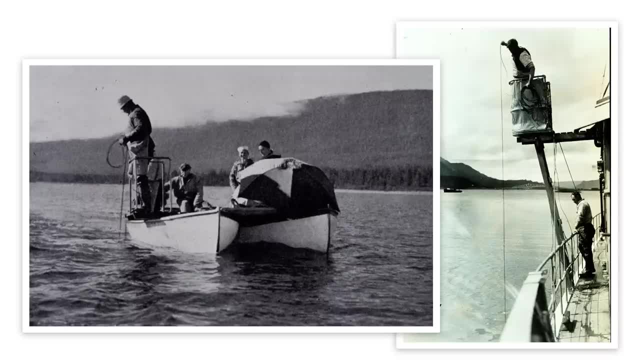 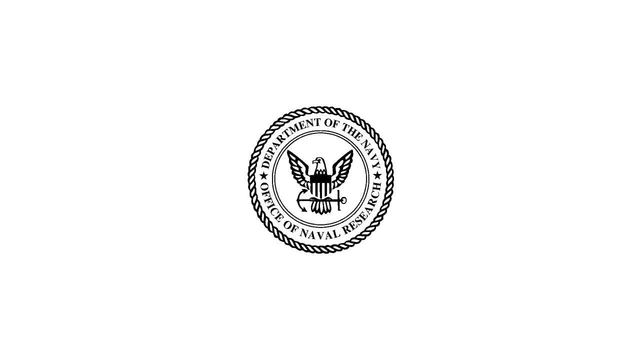 these maps were, as I mentioned, very crude and very limited and unreliable. But as World War I began and ended, and then eventually World War II came about, the United States launched a Department of the Navy, Office of Naval Research And, for the first time, 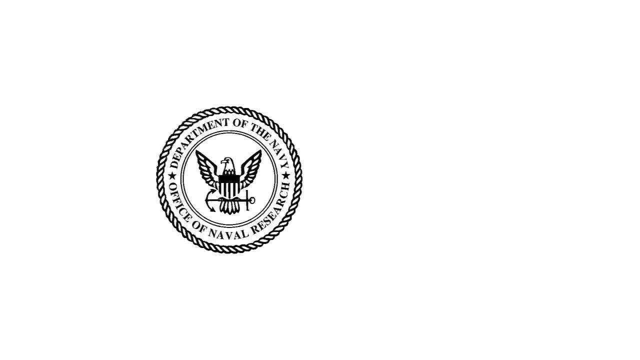 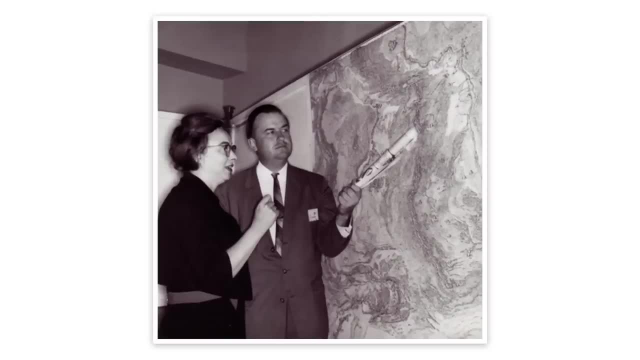 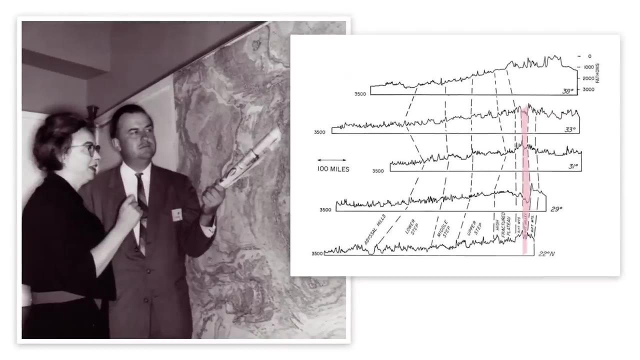 they launched a type of map that was driving an effort to map the ocean floor. In fact, scientists Marie Tharp and Bruce Heason developed the first bathymetric map of the Atlantic ocean, and this is in the 1950s. They used a technology known as sonar to map accurately the depth of 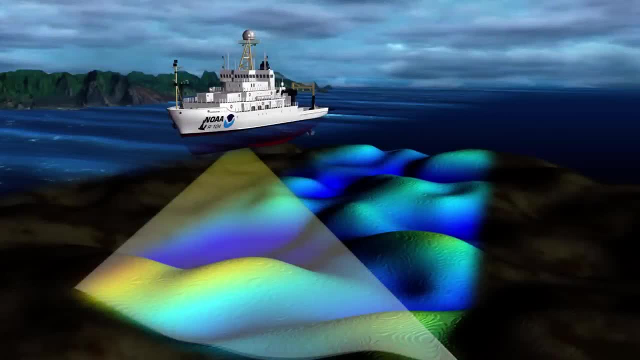 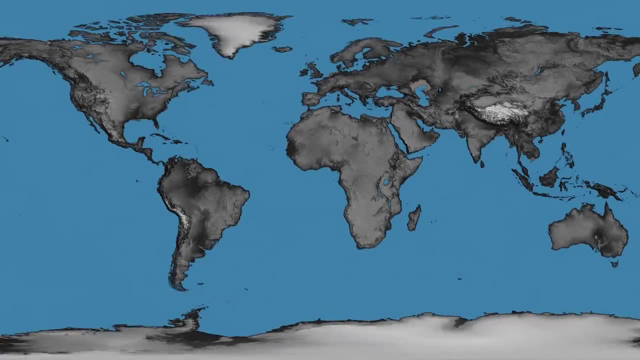 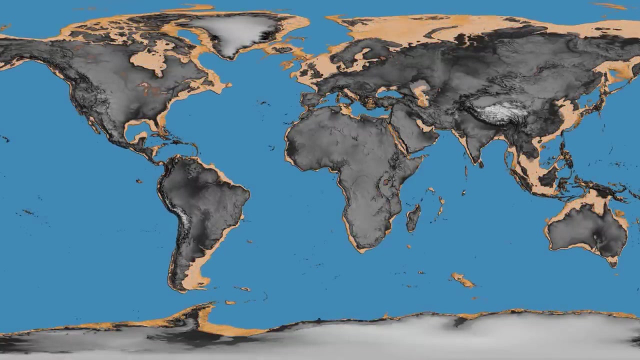 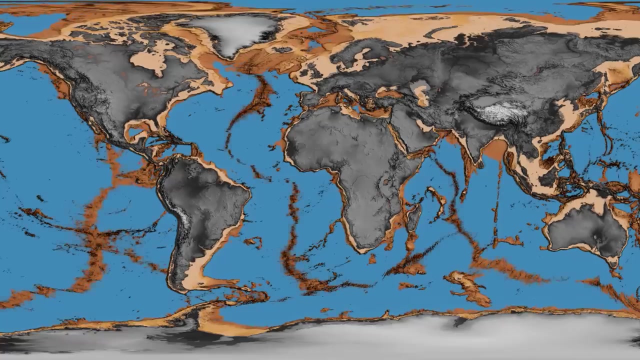 the sea over large areas, And they created a map that was the most accurate of its time, And so if take the blue oceans and drain them from the surface, what we would see is that the seafloor is not a vast expanse of flat desert, as was believed beforehand, but rather it was a jagged 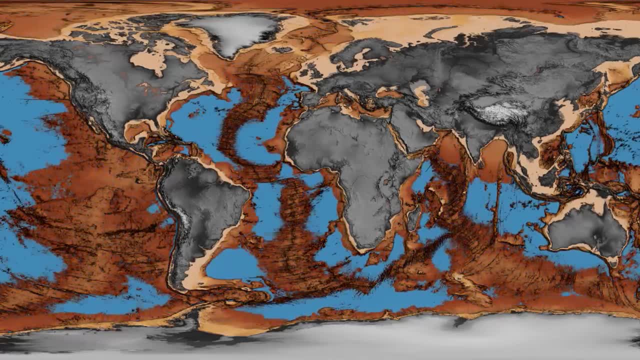 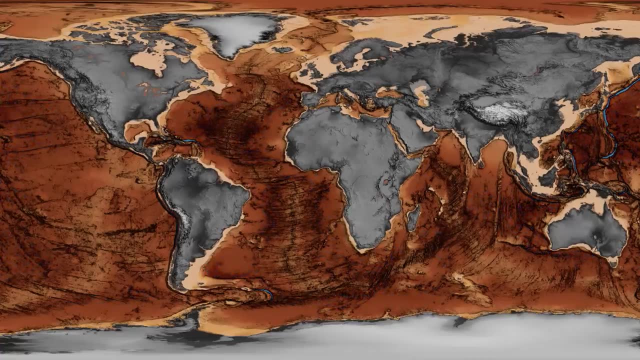 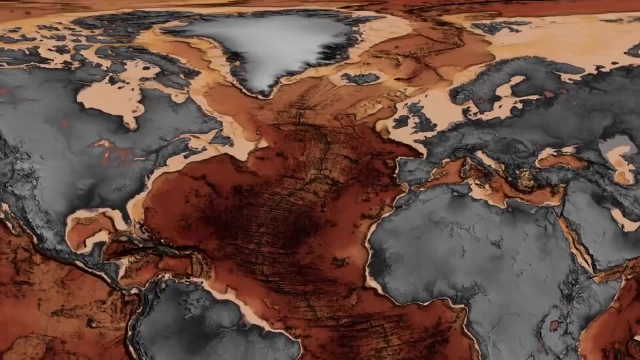 and active area with giant peaks and cracks, trenches, earthquakes and active volcanoes, as you can see here, now that we've drained out the water from the earth. If we zoom in on different areas, particularly the center of the North Atlantic Ocean and extending down through the 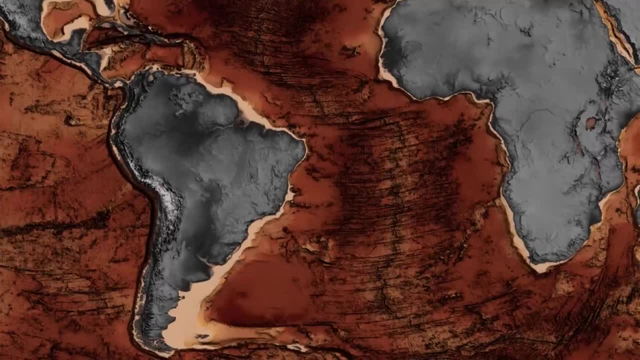 Southern Atlantic. you see this massive scar, this thousands of mile long mountain range that runs down the Atlantic Ocean basin and essentially mimics the shape of the continents. This set off some alarm bells and, as you can see, the seafloor is not a vast expanse of flat desert, as was believed. 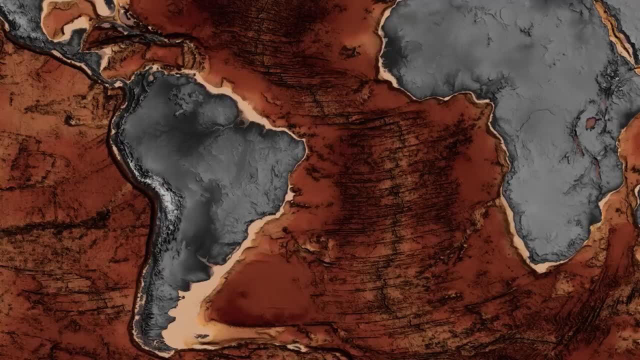 beforehand, but rather it was a massive set off some alarm bells and, as you can see, the seafloor is not a vast expanse of flat desert as was believed for scientists, as they believed that this could potentially be related to Wegener's earlier theory of the moving continents. 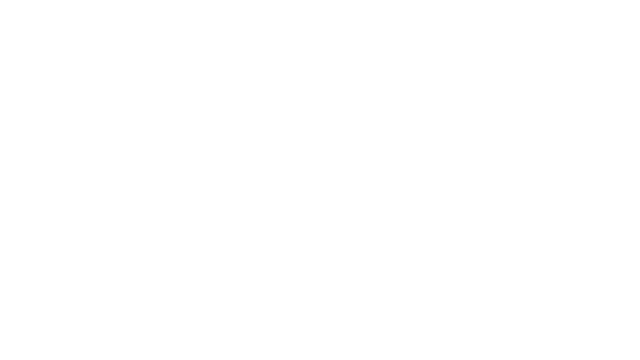 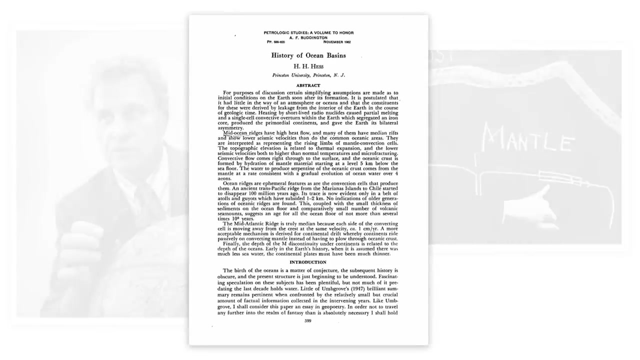 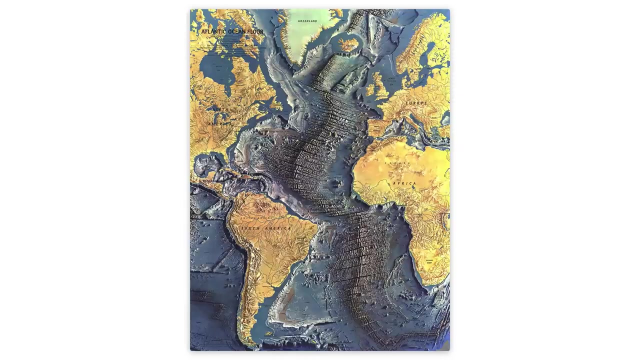 After the work of Tharp and Heason came along other notable scientists, including Robert Dietz and Harry Hess, who published work that further described the fascinating geological structures that are found in the bottom of the ocean. In fact, if you were to draw a profile from North America to Europe, you would see something like this, with: 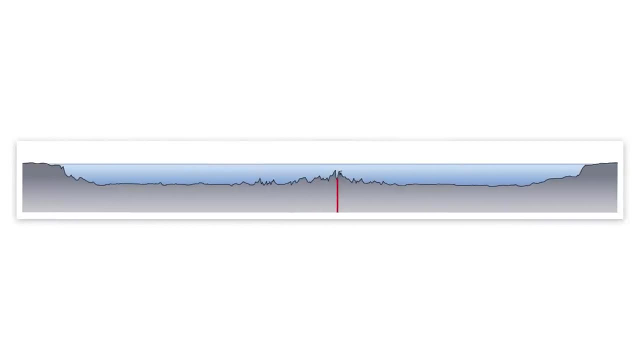 vast expanses of flat areas and then that jagged, irregular central mountain range that runs down the center of the Atlantic Ocean. And so this simple observation that the seafloor has geology became supporting evidence number one. So there are active fractures in the lithosphere or the 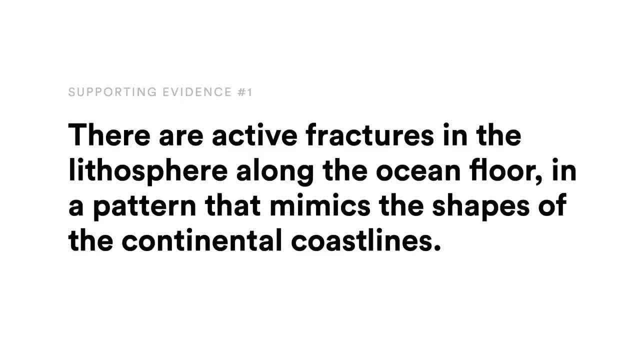 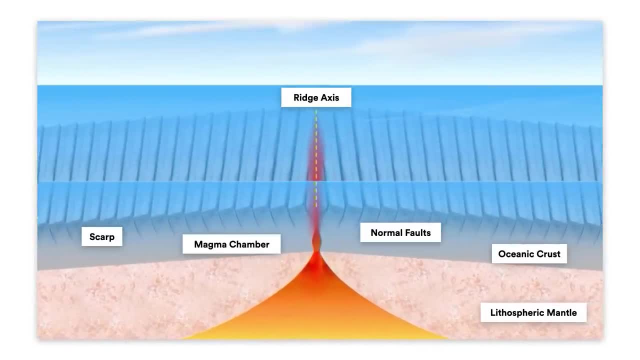 crust of the ocean floor in a pattern that appears to mimic the shape of the continental coastlines. Based on these observations, scientists like Hess developed an idea that, along this ridge, magma from underground magma chambers was spewing up through the crack in the Earth's surface. 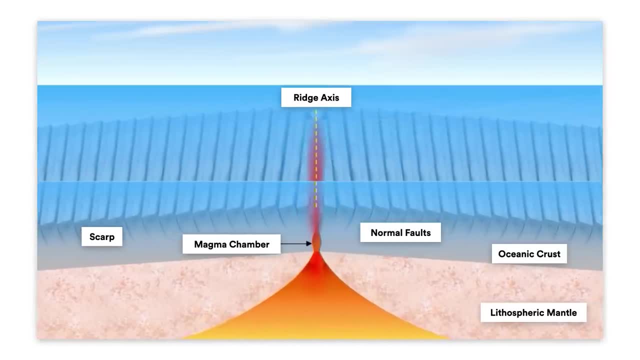 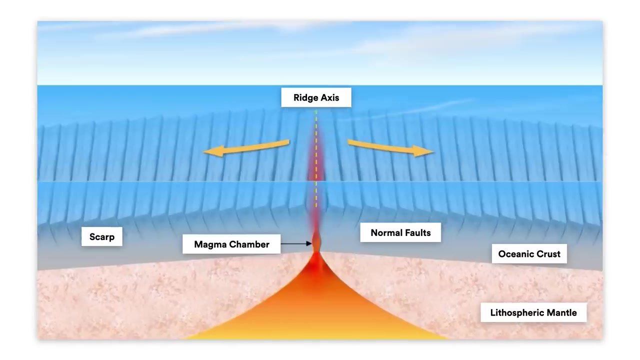 and pushing the plates apart, pushing the slabs of rock on either side away from one another in what would become known as a spreading center or a divergent plate boundary, as seen in this animation here. Slowly, over time, the plates spread apart, carrying the rock and the sediment with them. 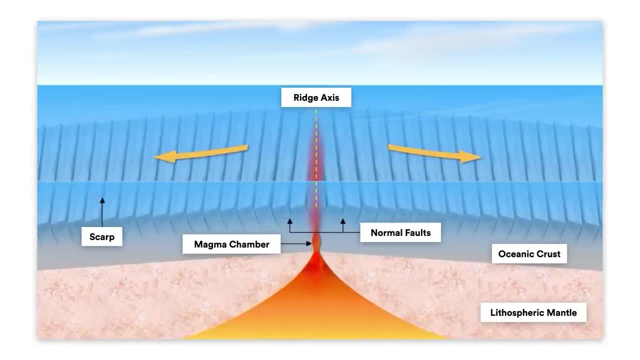 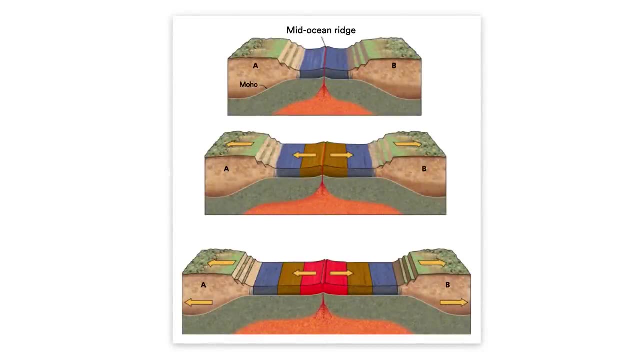 And along this boundary we see lots of cracks, called faults, and scarps in the surface of the Earth. Here's another diagram that illustrates what we think happens along these spreading centers where magma pushes its way through the earth. It pushes its way up through the crack and spreads the plates apart above. 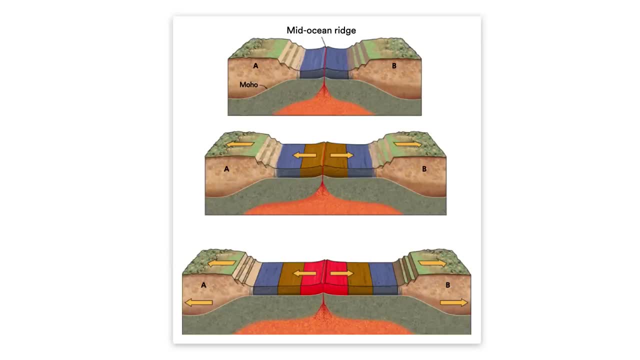 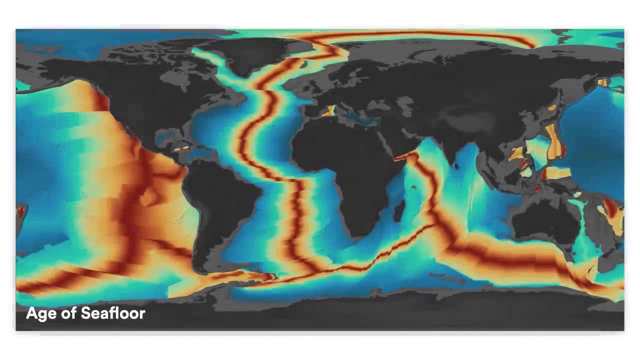 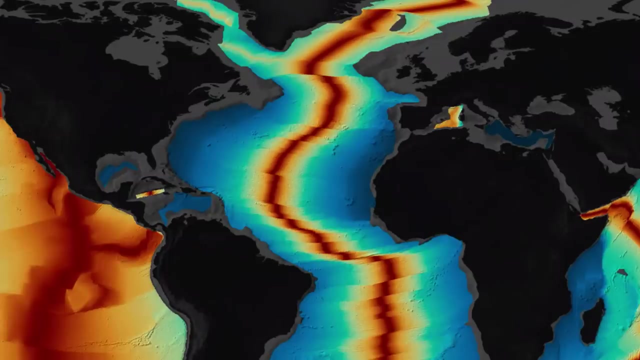 And so one of the ideas was to look at how old the rock on the seafloor is, as that could potentially support this notion. And if you were to map the age of the seafloor, similar to what we see here, what you would notice is that, shown in red, we have very young rock right along the ridge. 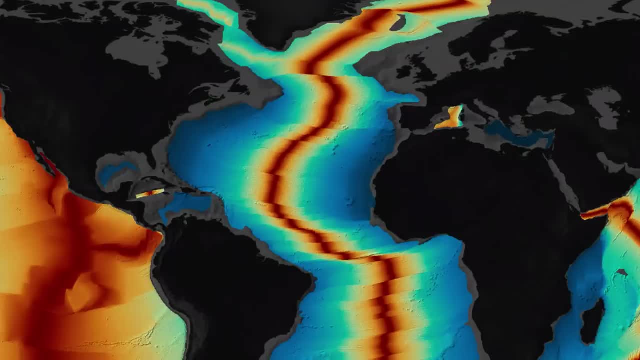 And then as you go away from the ridge in either direction, through the ore, from the orange and yellow to the green and then blue, the age of the seafloor gets older, And so the only way that's really possible is if, in fact, seafloor spreading is occurring. 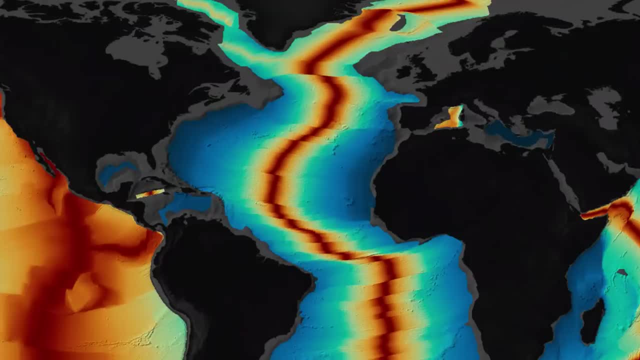 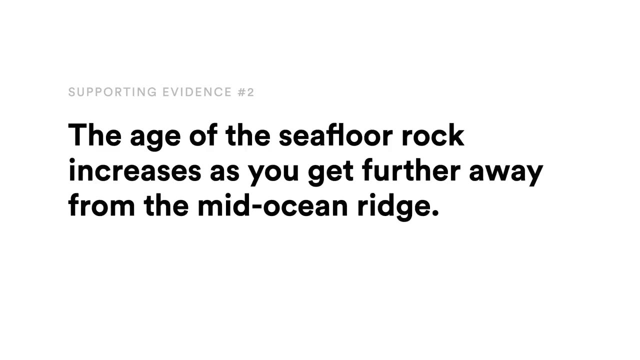 and that Harry Hess and other scientists were correct in their theories. So supporting evidence number two is that the age of the seafloor rock increases as you get further away from the mid-ocean ridge, But as you go away from the mid-ocean ridge. as you get further away from the mid-ocean ridge. 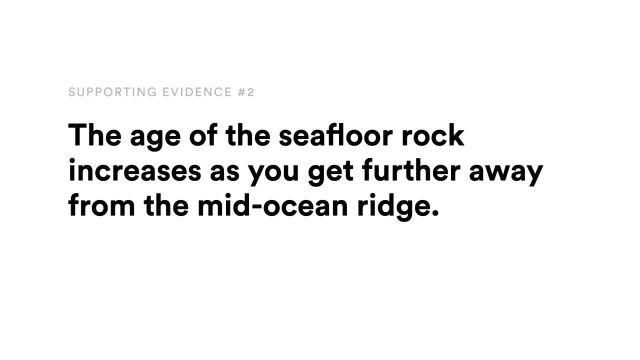 But as you go away from the mid-ocean ridge, as you get further away from the mid-ocean ridge, as with all science, we're constantly looking for more supporting evidence, And so scientists went back to the drawing board and they thought about other things that could prove that this is in fact happening. 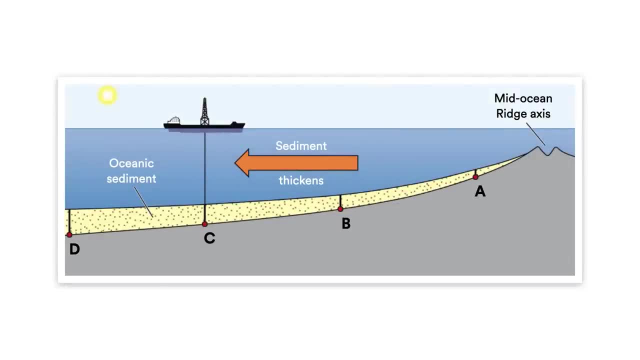 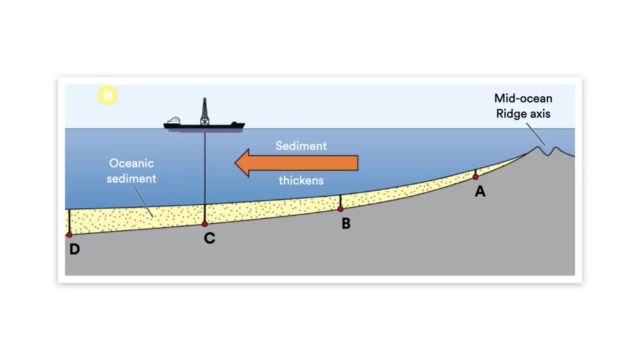 and old rock should be found further away. scientists believe that sediments should become thicker in their layers as you get further from the ridges, which makes sense, because older rock would have had more time to accumulate sediment, as you can see in this diagram. 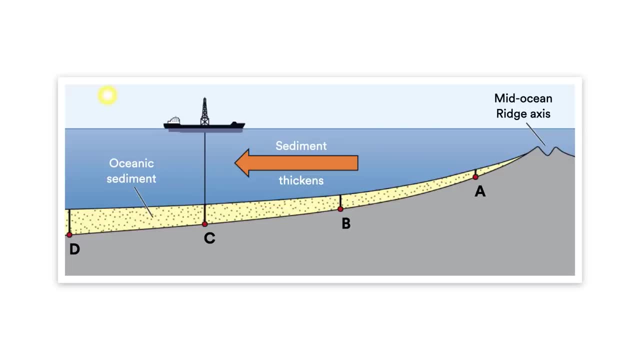 If you were to travel along the seafloor from point A to B to C to D, you would notice that that layer of sediment increases in its thickness. you would notice that that layer of sediment increases in its thickness. you would notice that that layer of sediment increases in its thickness. 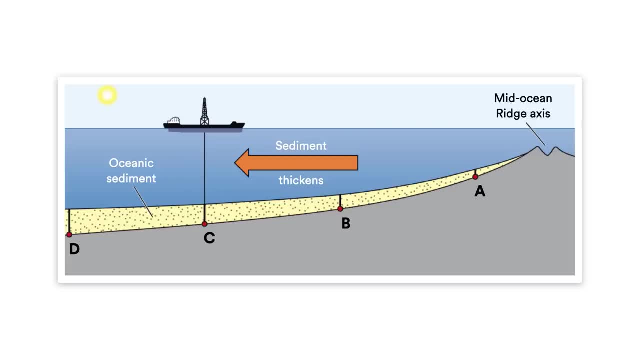 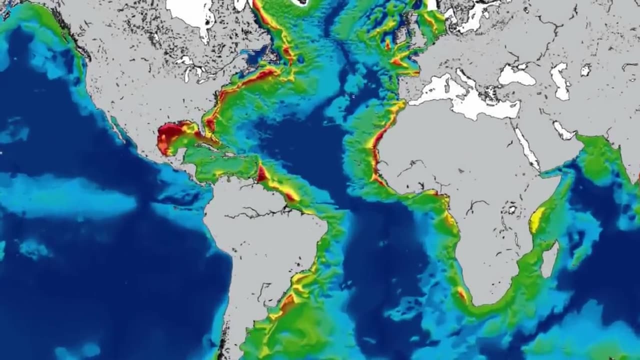 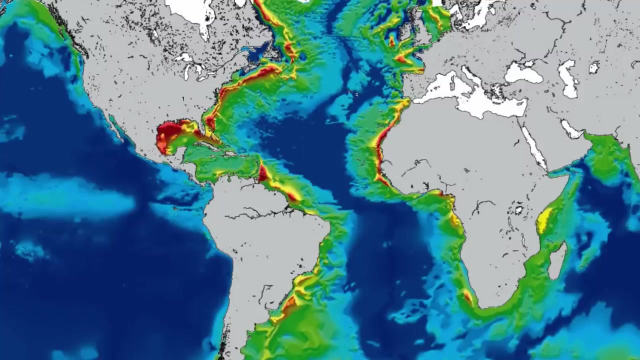 And that's because the rock is older and there has been more time for the accumulation of that sediment. And this proved to be true as we studied the seafloor more and more, as with this map showing sediment thickness with different colors, with the dark blue being thin layers of sediment. 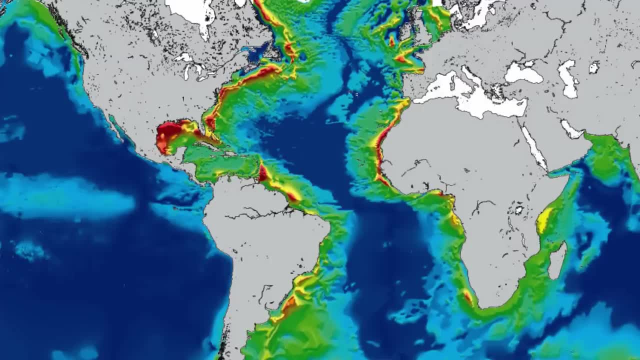 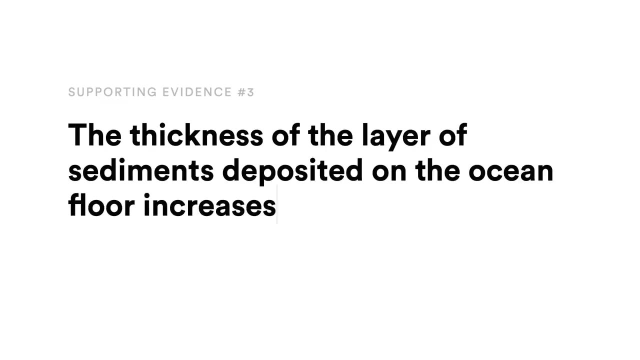 and light blue, to green, to yellow and red, becoming thicker and thicker. And so that gives us supporting evidence number three. and so that gives us supporting evidence number three that the thickness of the layer of sediments deposited on the ocean floor increases as you get further away from a mid-ocean ridge. 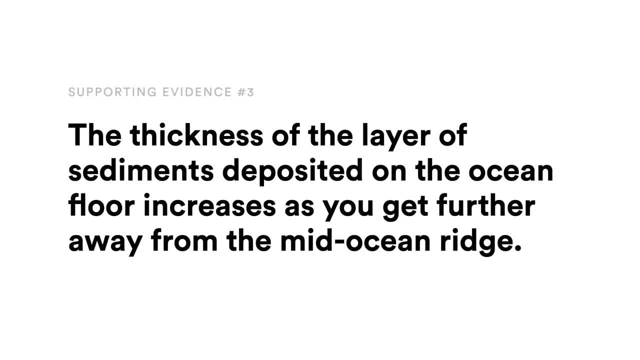 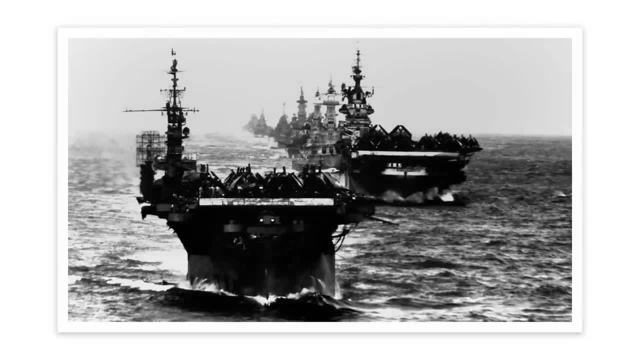 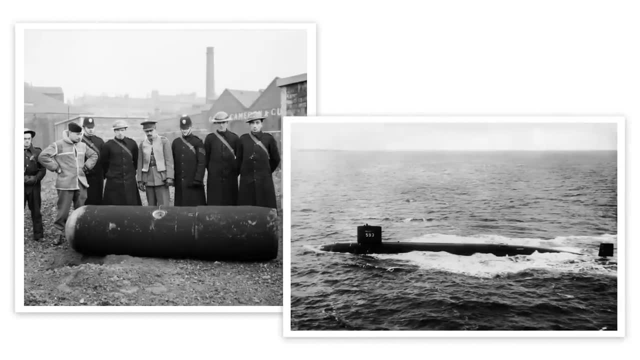 And so, once again, we would look to warfare and the Navy to get more scientific information to support the concept. Now, during World War II, one of the issues that the Americans and our allies were dealing with was being able to identify these massive sea mines and submarines that were being used. 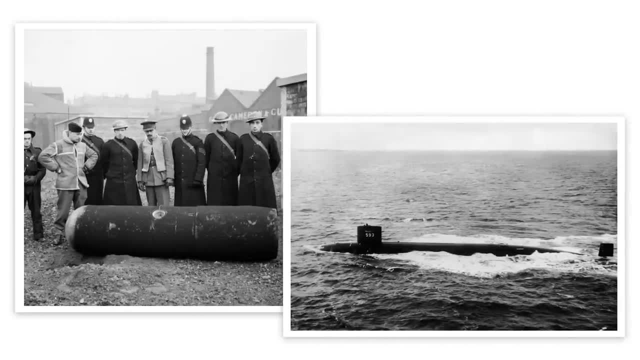 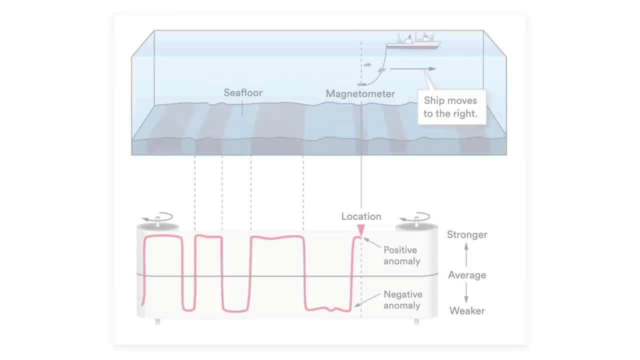 was being able to identify these massive sea mines and submarines that were being used by the Germans, And so one thing we did was begin to study magnetism Using new technology. we could travel across the ocean in a boat or in an airplane and detect the magnetic field under the ocean surface. 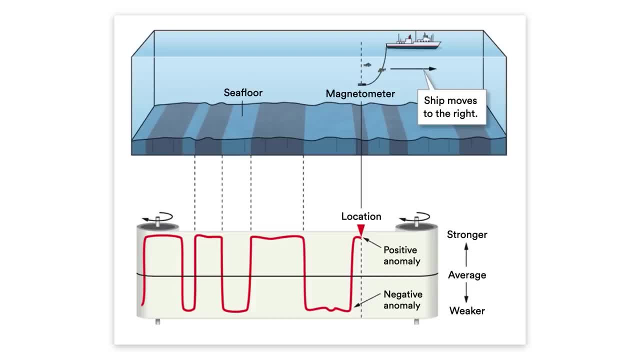 Now, submarines and mines give off a certain amount of magnetism or are sensed by this equipment, and so we are able to actually detect them, even if they're out of visible sight. But we also were able to detect magnetism of the sea floor. 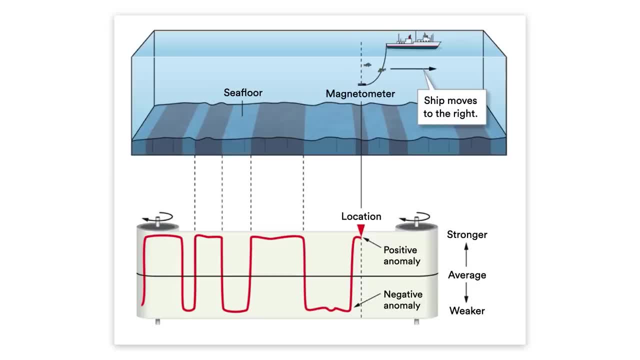 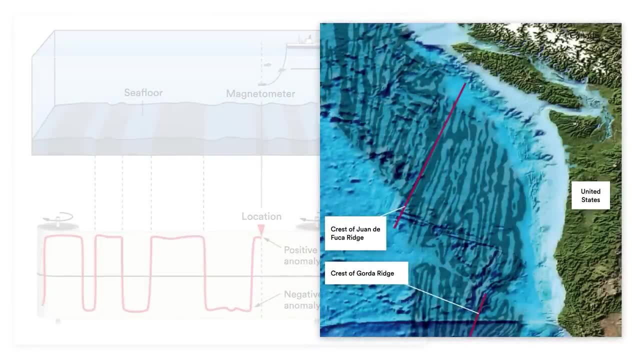 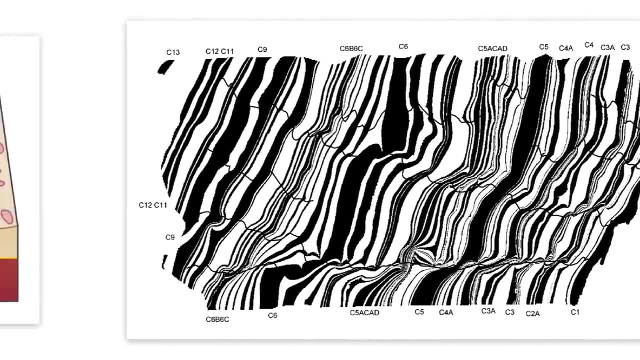 and we found something fascinating, which is that if you look at the magnetism of the sea floor in different areas, it's not random as you might expect, but rather you see these bands or stripes of alternating magnetism, as seen in this diagram or this one here. 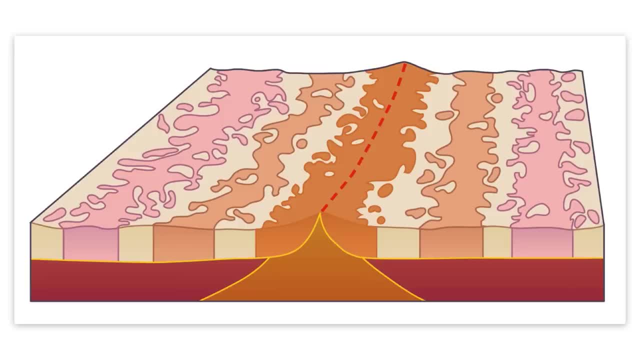 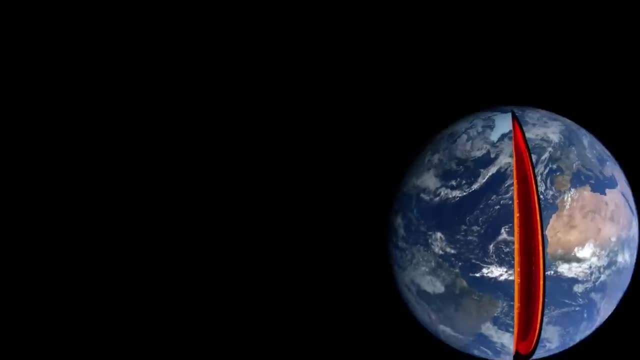 Now, in order to really understand this, we need to step back a little bit and actually look at the magnetic field. Let's look at the inside of the Earth. In case you were unaware, the inside of the Earth is made up of different layers. 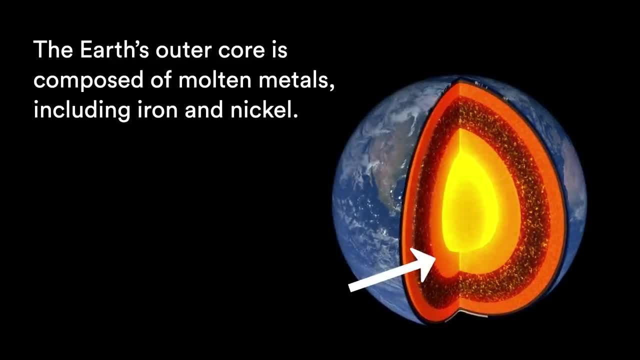 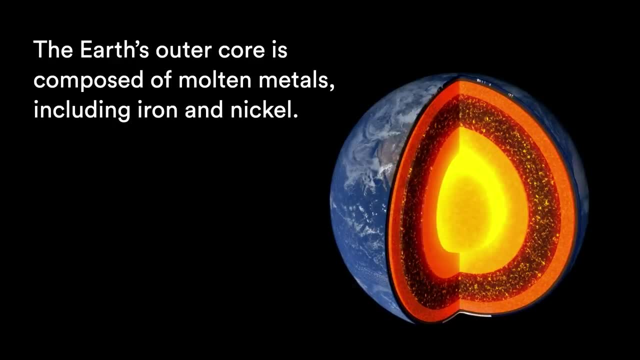 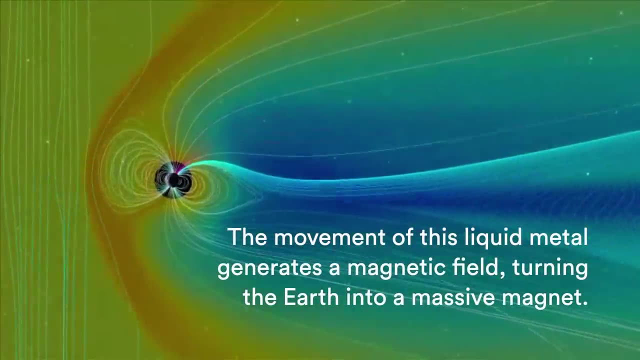 and one of those layers, the outer core shown here in orange, is composed of molten metals, including iron and nickel. Now, those molten liquid metals are not sitting still, but rather they are flowing around the inner core, and the movement of that liquid metal generates a magnetic field. 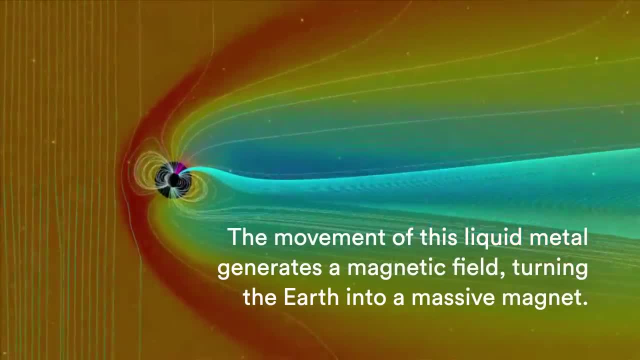 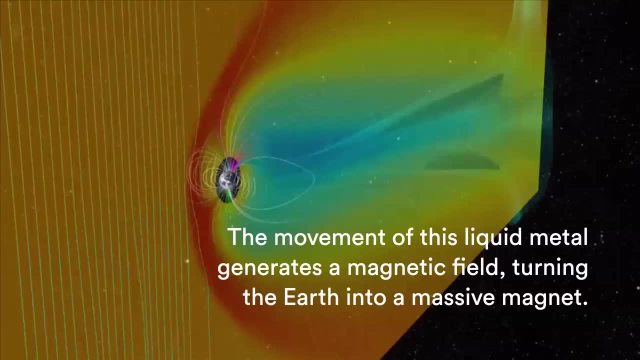 which essentially turns the Earth into one gigantic magnet. Now, the fact that the Earth is a magnet and has a magnetic field is very important for a lot of different reasons which we won't get into in this video, but it's important that you know the Earth essentially is a magnet. 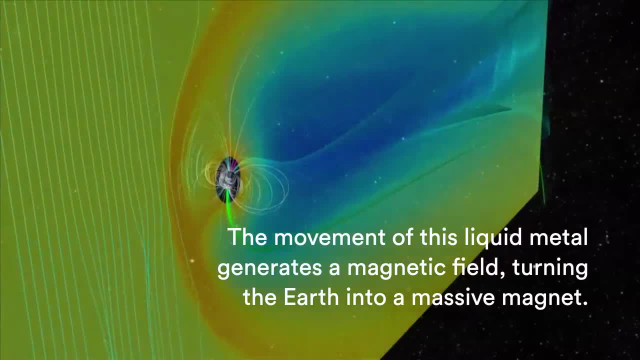 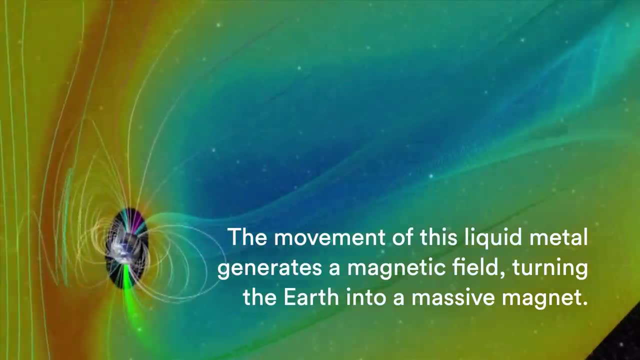 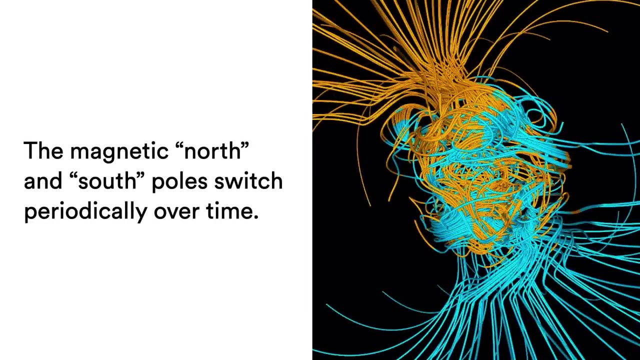 And, just like a magnet that you would play with, it has both a north and a south pole that behave a little bit differently and are detectable. Now, a strange phenomenon we have seen on Earth is that the magnetic north and south poles- the south poles- switch periodically over time. 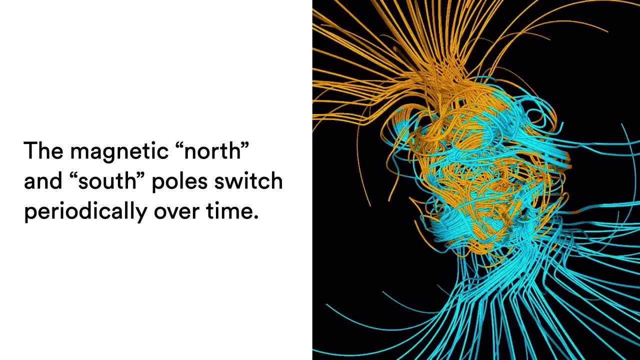 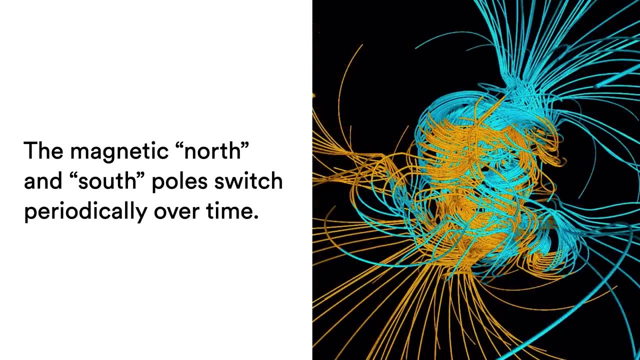 So if you look at this visualization, let's say that the orange area represents the magnetic north and the blue represents the magnetic south. Now, over time those poles will become kind of all haywire and then eventually flip, so that north has become south and south has become north. 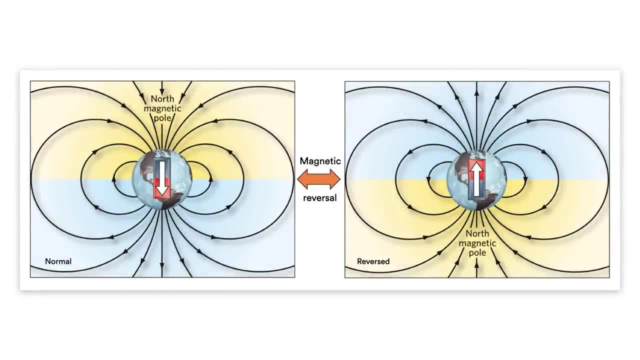 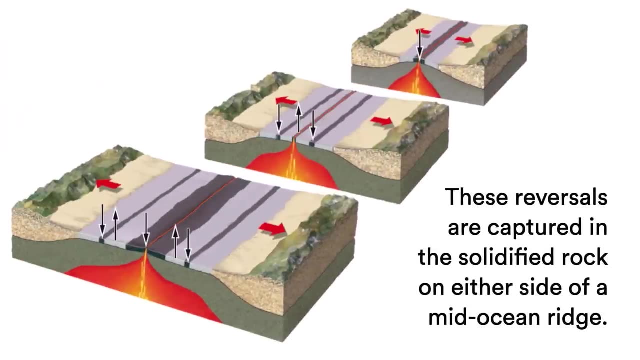 This is known as a magnetic reversal, and we see it happen on a fairly regular time scale throughout Earth's geologic history. Now here's why this is so important and relevant to seafloor spreading: It's because these magnetic reversals are captured in the solidified rock. 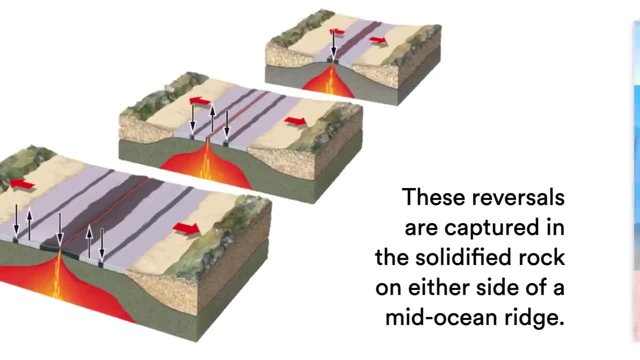 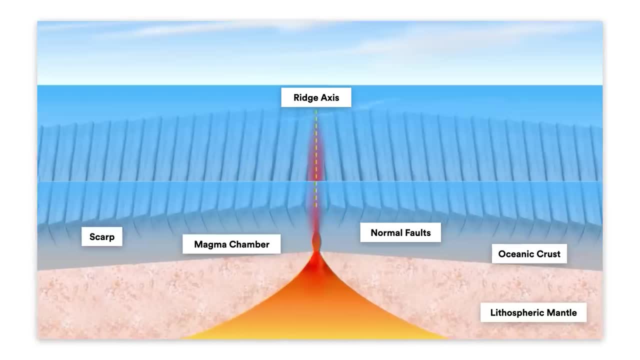 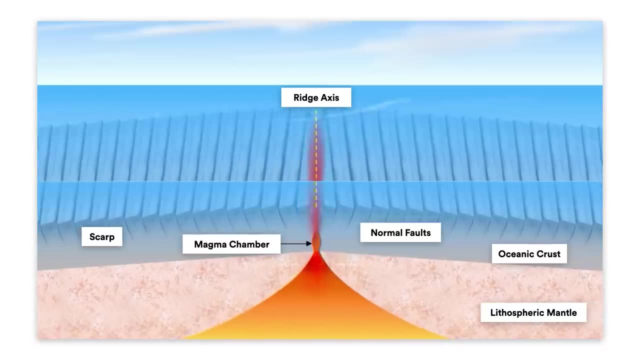 on either side of a mid-ocean ridge. As magma wells up through the ridge and hits that cold ocean water and solidifies into rock minerals within the magma, align with the Earth's magnetism, which is the magnetic field, And then we forever have a record. 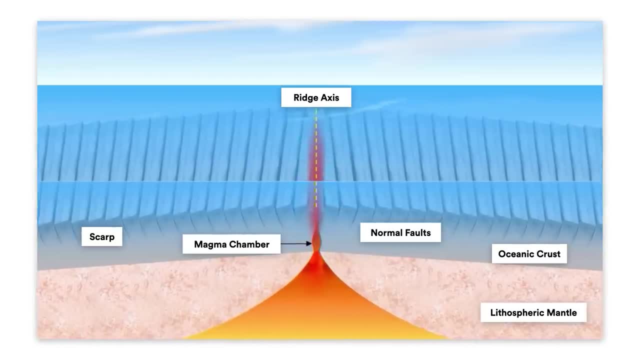 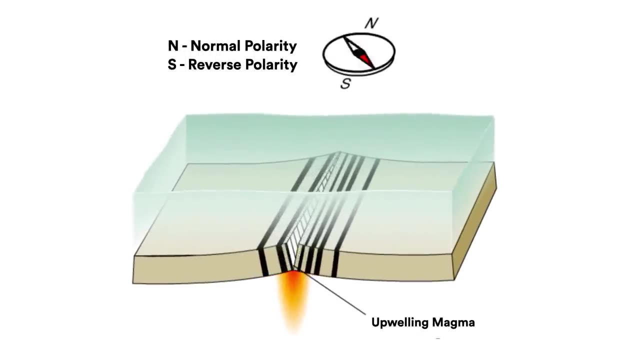 of what the Earth's magnetic field was at the moment that that rock formed. Let's look at this animation, which shows it clearly that, as magma upwells and solidifies, it records the Earth's magnetic field And whenever those switches occur. 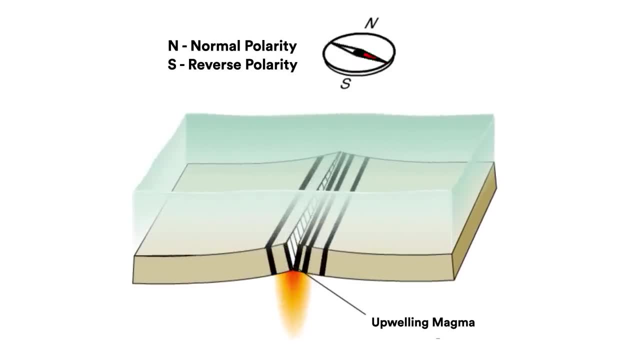 we see it as a record within the rock. Now it's shown here with different colors, but it's not the case in reality. However, if we could see the seafloor magnetism, we would see patterns that look kind of like this: 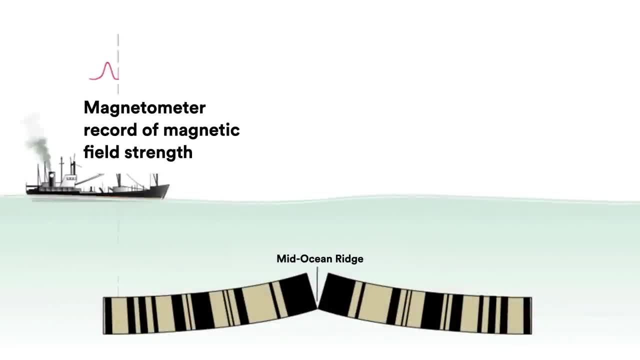 If we were to come back over this area with a boat and measure it, what we would see is that the pattern of magnetism matches up perfectly on either side of the ridge. Where we see positive magnetism on the left side, it aligns with a similar band on the opposite side. 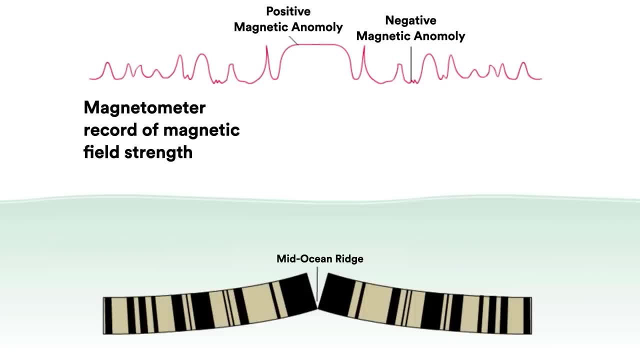 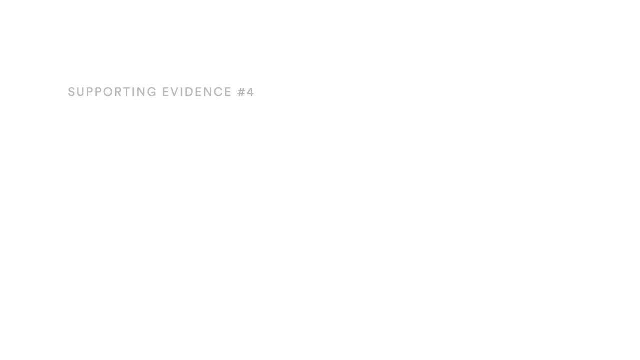 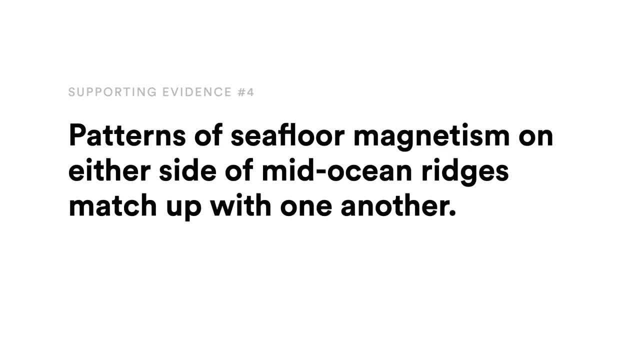 And the only possible way that this pattern could exist is if the seafloor is spreading, And so this becomes supporting evidence. number four Patterns of seafloor magnetism on either side of a mid-ocean ridge matches up with one another, And so this gives us a complete case. 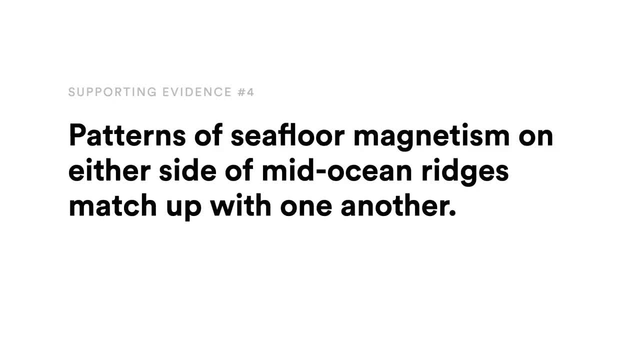 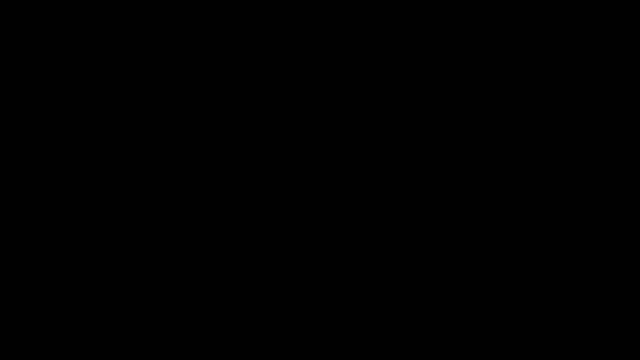 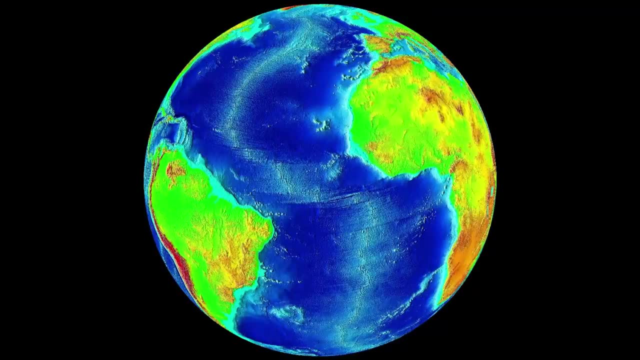 that proves that the seafloor on Earth is in fact spreading apart and that plate tectonics is a real phenomenon. So when we look at the Earth and we see these fascinating structures under the ocean, we now understand why. All we have to do is look at these.